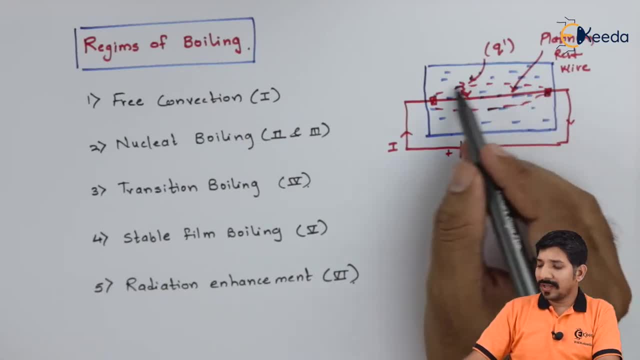 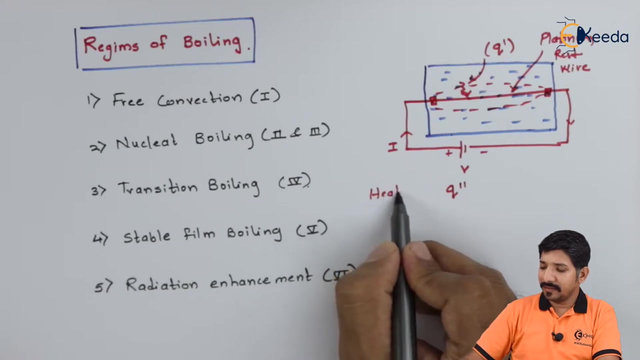 critical heat flux occur. So for that what they have done, they have kept the notation of the heat flux. So heat flux is indicated by q double dot. So let me write: this is heat flux, which is nothing but the rate of heat transfer per unit area. The unit for the same is watt per meter square. 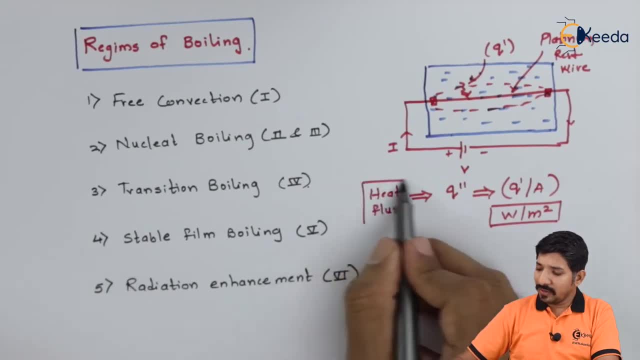 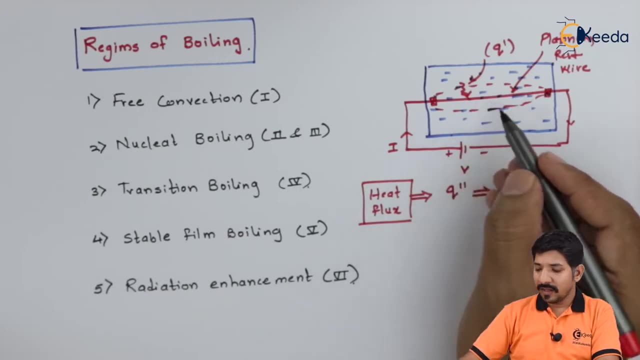 So what they have done is they have tried to find out what is the amount of heat flux that is going through the wire at a particular length with respect to the change in temperature. Now, remember this: they have considered the change in temperature. The change in temperature is nothing. 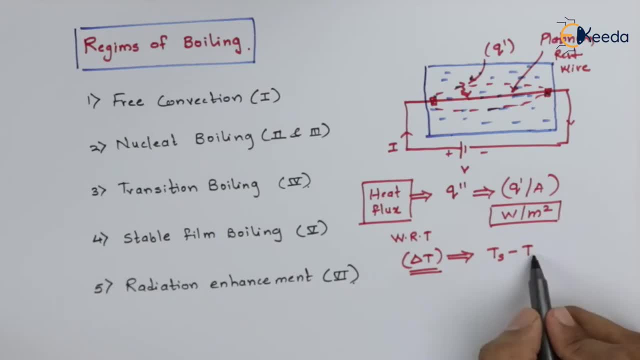 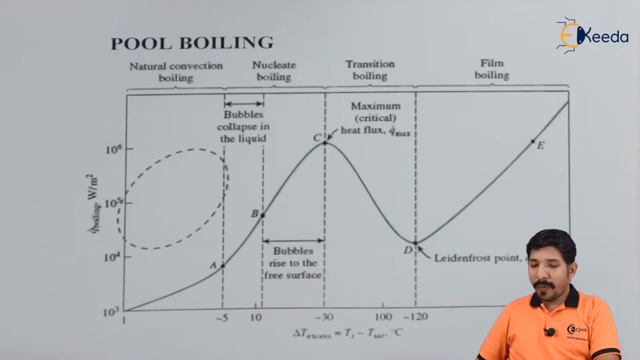 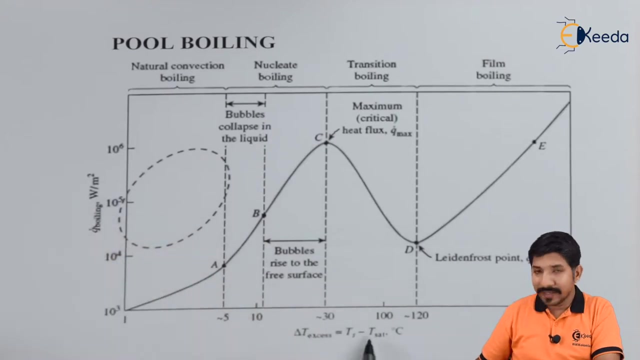 but the surface temperature minus the wire temperature, or the surface temperature minus the saturated temperature. Now this T sat is nothing but the saturation temperature of the given fluid. So by doing so, what they have observed is the variation of heat flux with respect to temperature. the profile looks something like this. Now, what they have done? they have 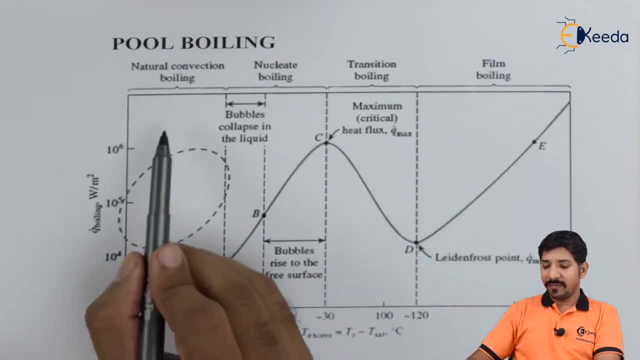 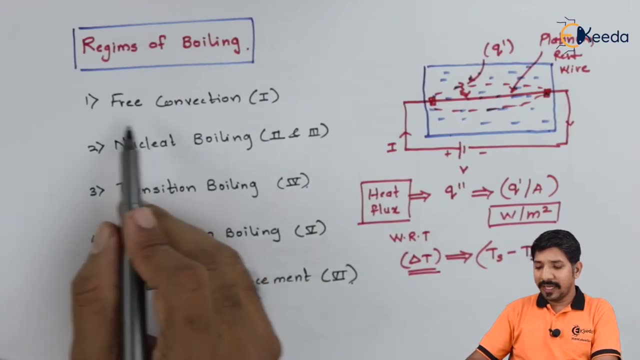 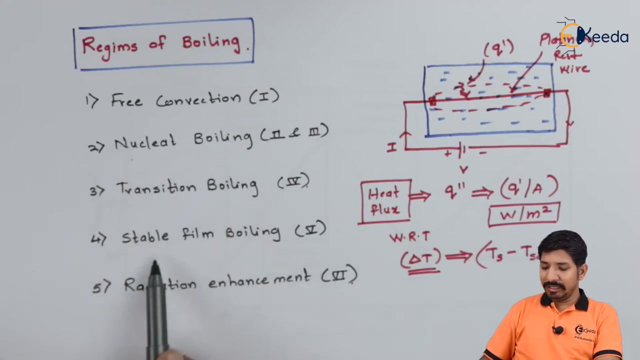 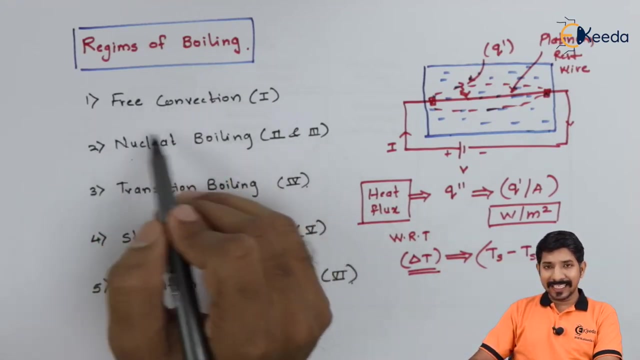 tried to categorise this profile within five categories. The first one is natural convection. now categorise the same in free convection or the natural convection, then the nucleate boiling, then the transition boiling, then stable film boiling and radiation enhancement, So corresponding to the category or the regime. 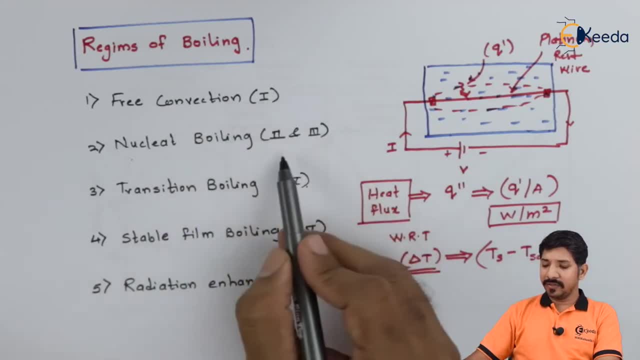 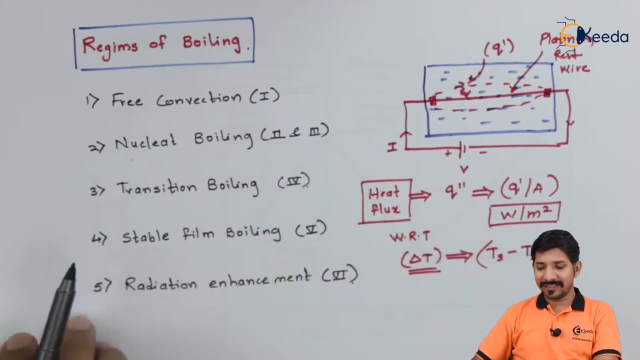 they call it. we have given the name, now this: 1, 2, 3.. Now these are the names which are there, given in the diagram itself. So let us look at the diagram to understand it. So in the diagram, as you can see, till 1 to 5.. 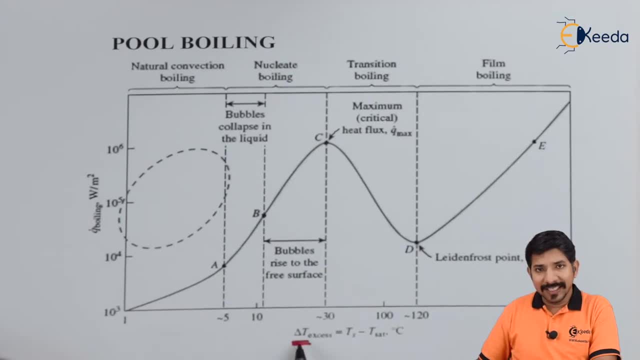 Now 1 to 5 talks about the delta T till the change in temperature. stays within 5, the heat transfer rate is entirely natural. So here there is no phase transfer. all the heat transfer rate is by free convection itself. So let us write down here: this is free convection or natural convection. 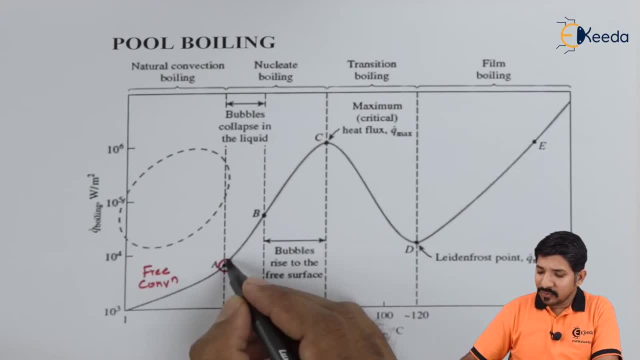 Now what happens at point 1. as I reach to point 1, the bubbles will start forming. The first bubble will be formed approximately at 5 degree Celsius delta T. Now, from 1 to 2, the bubbles will keep on forming onto the wire. 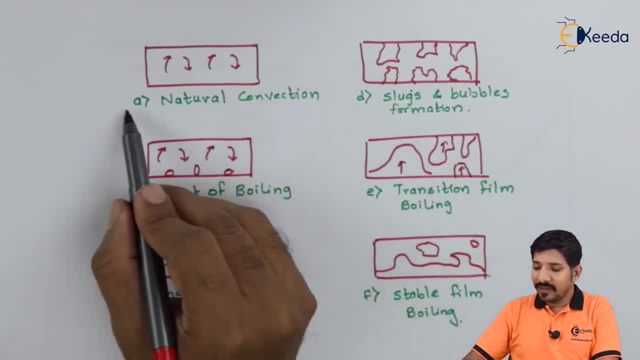 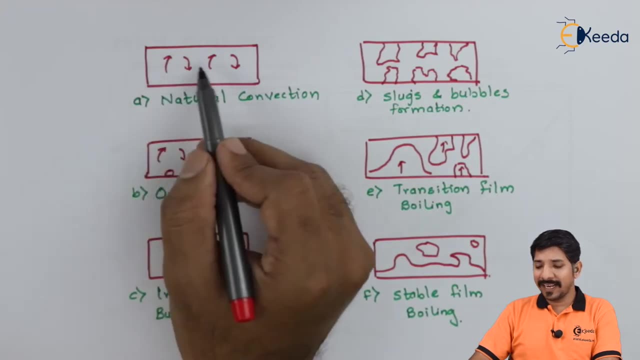 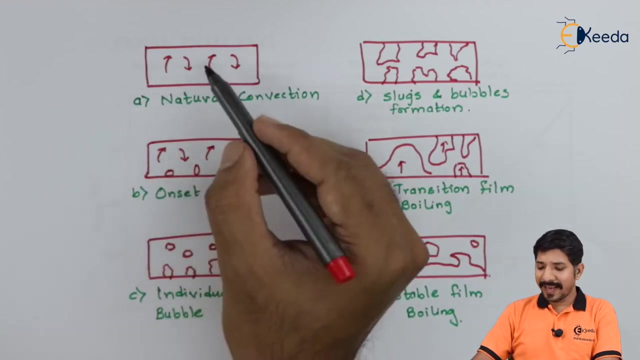 See, it can be seen with the help of this diagram itself. The first one was natural convection. Here, simply, a hot fluid is getting upward because of the change in density and the colder fluid was going downward. So this way, till the 5 degree Celsius, the natural convection takes place, and then, second, 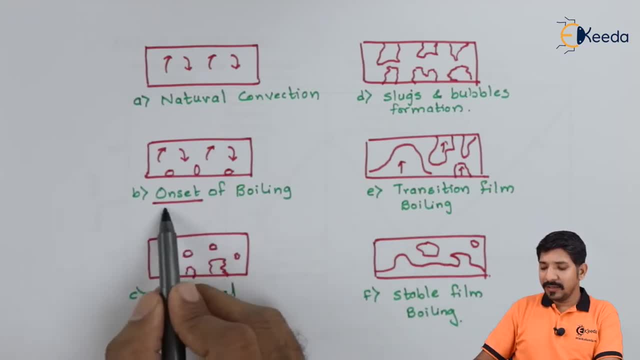 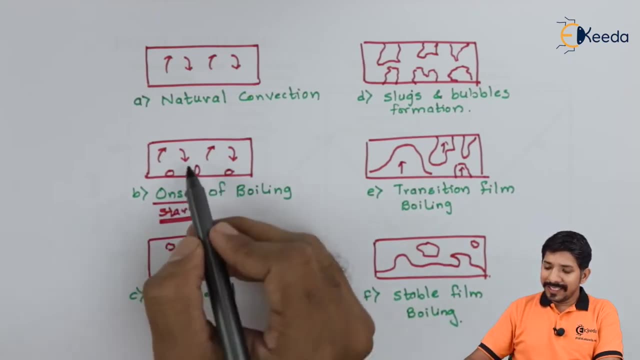 comes the onset of nuclear boiling. Now, onset is nothing but the start. So this is nothing but the start of nuclear boiling. So in this, what is happening? the small bubbles will be formed onto the surface, But mind it That in this region the bubbles will never detach itself from the surface. 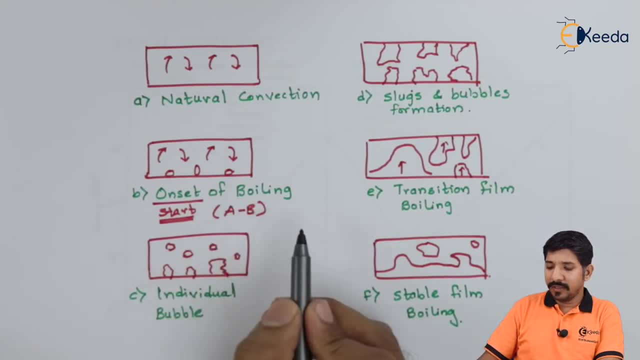 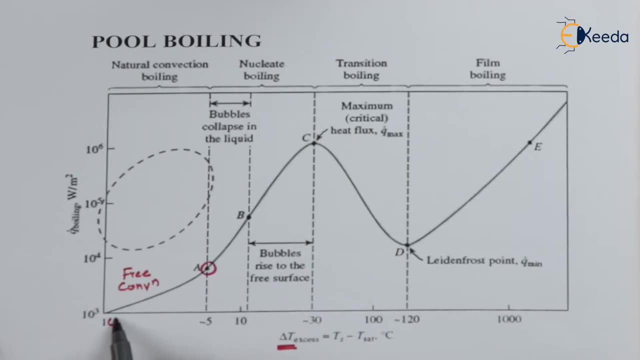 Now this region is what they call is from A to B, And this region I can say that it is from. let's say O to B. See if I call this point O. So O to A is nothing but your free convection and A to B is your onset of nuclear boiling. 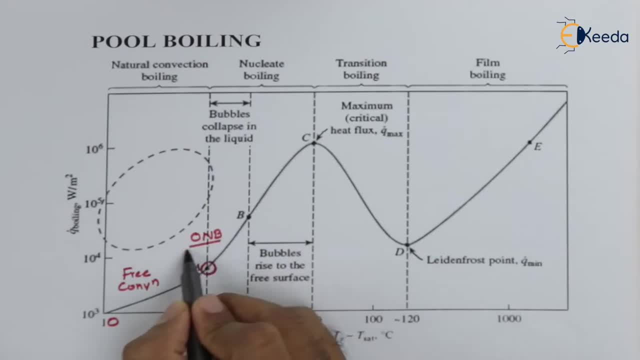 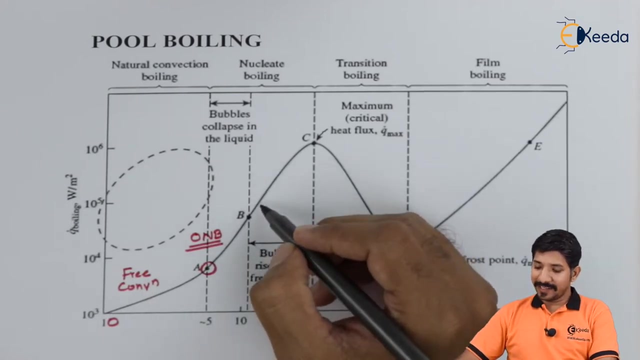 So they call O and B Onset of nuclear boiling. Then what happens after that If I still keep on increasing the delta T, as we can see that this point B is somewhere between 10.. Now what happens after that If I still keep on increasing the temperature? 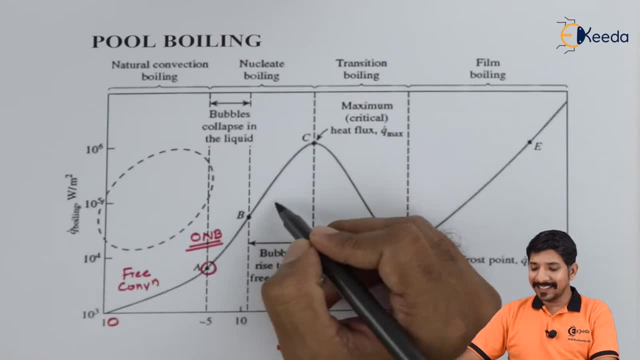 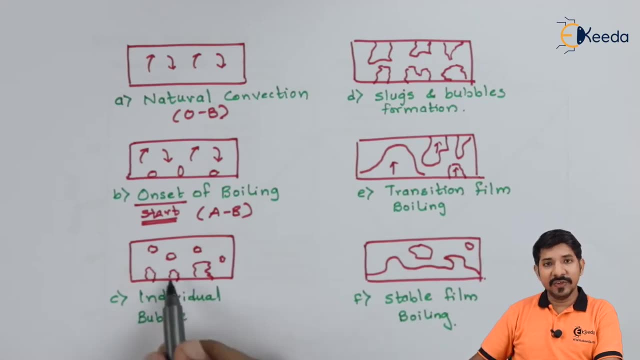 The bubbles will start growing and then they will start detaching the surface. See here, as we can see, this is the region which is basically the individual bubbles will be formed, They will start detaching from the surface and then they will start growing upward. 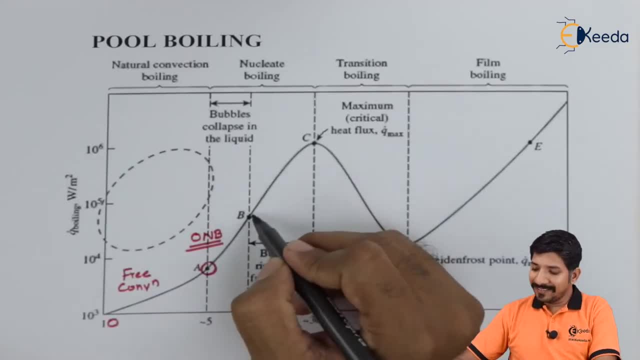 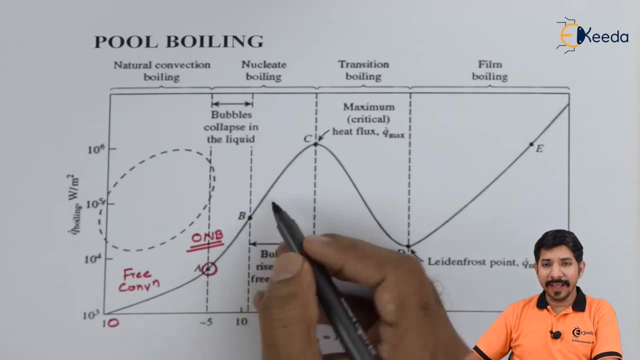 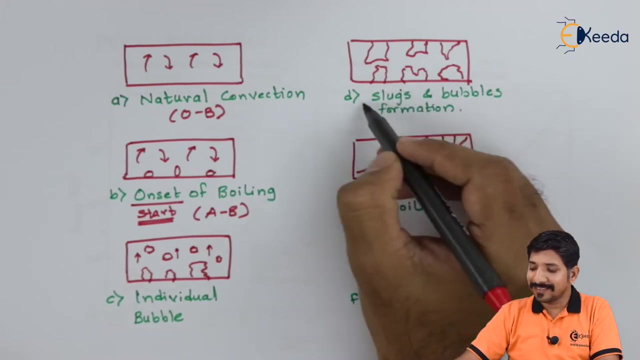 Now, this is your actual nuclear boiling. Now, in this case, this region comes around point B. So around point B the bubble will start forming and then it will start going in the upward direction. Next is the sludges and bubble formation. Now, what do you mean by the sludges? 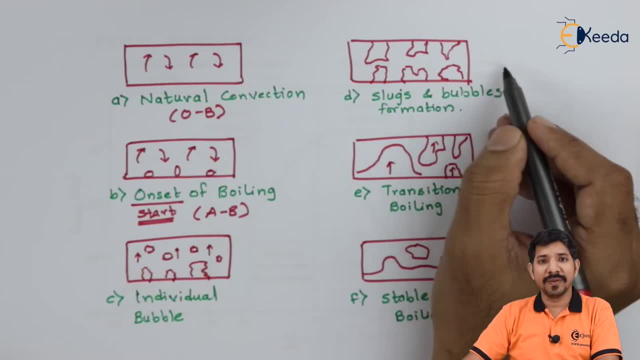 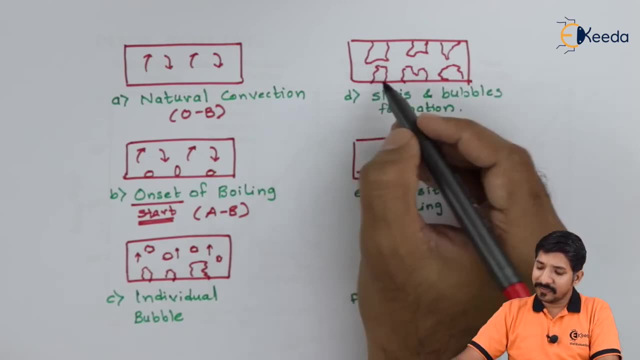 Sludges are nothing but the combination of many bubbles. So they are. They can be called as bigger bubbles if you want, But what is happening in this region? In this region, if you can see that a lot of area is vacant due to the sludge bubble, which 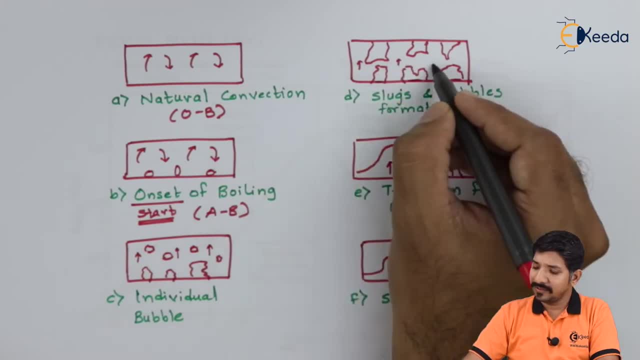 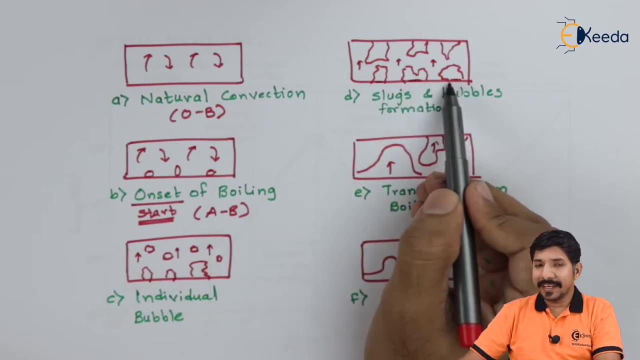 are formed and again they have started moving in the upward direction. Now, these small area which are formed due to the sludges, They have created a area for the heat transfer rate. Now, because of this small area that is created by the sludges, 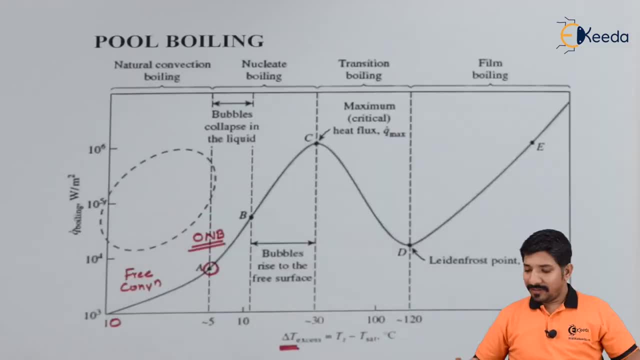 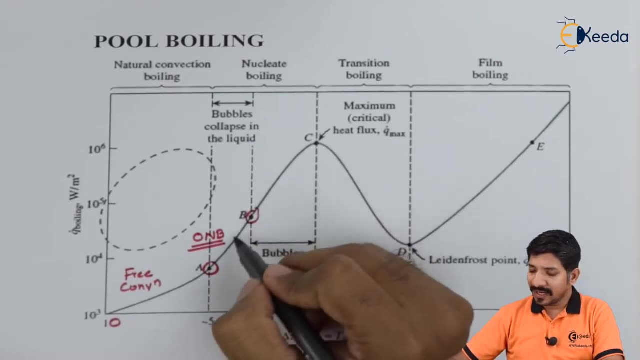 They have created a And the heat transfer rate may get enhanced. See, the same can be seen here. from A to B We have the onset of Nuclear boiling. then around B to C We have the actual nuclear boiling, where the bubbles have formed and then they have accumulated. 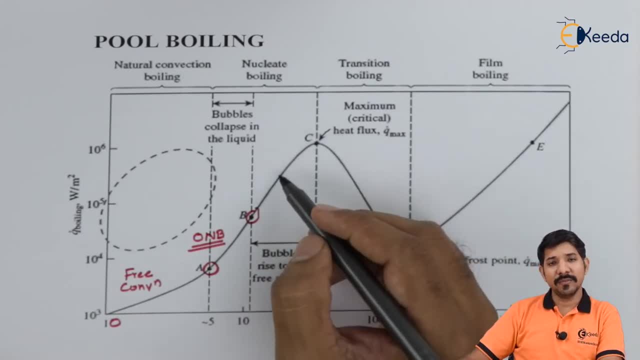 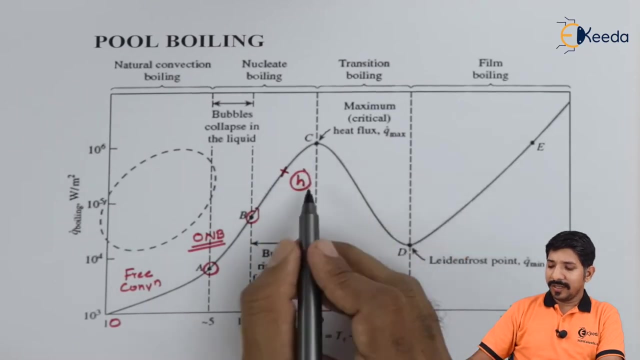 themselves to form from the sludges and then they have started moving in the upward direction. Now, because of this, What is happening? that in this region, somewhere around here, The value of heat transfer coefficient is is the maximum. So what we want- that the heat transfer coefficient to be maximum. we. 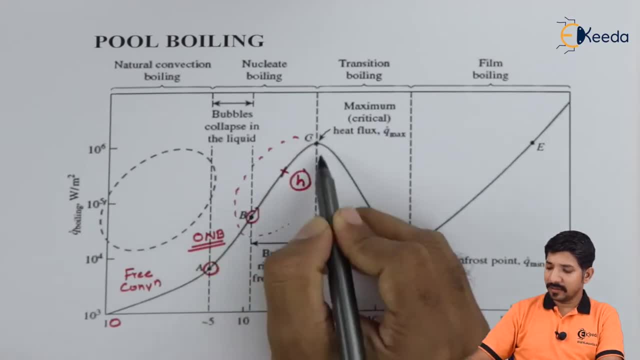 should stay near this region. So this region is what they call as the prime for the nuclear boil. But the difficulty for this region is that of point C. Now let us understand what we mean by point C. The point C is, as you can see, as I keep on increasing the delta, 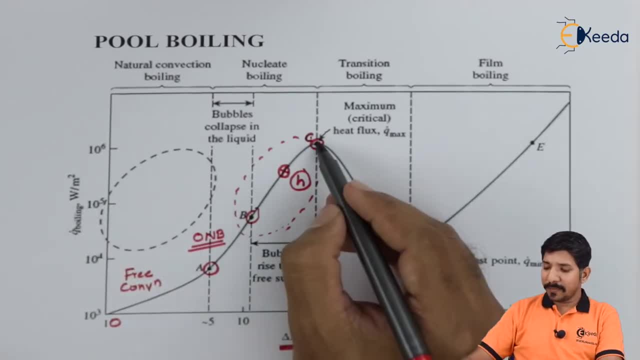 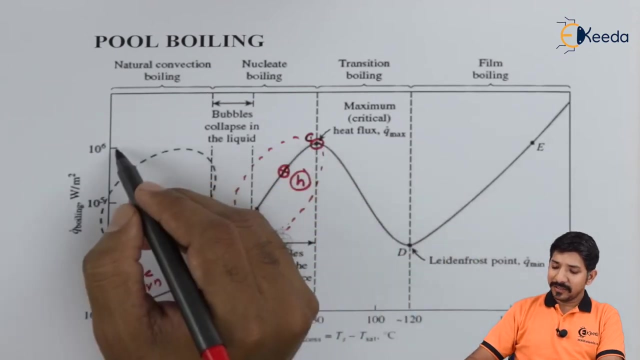 T, my value of Q start increasing. but there comes a point. let us say it is in case of water and the platinum wire, the experiment that was conducted. If I reach to around 30 degree Celsius, we reach to point C. Now what is happening at point C? At point C? 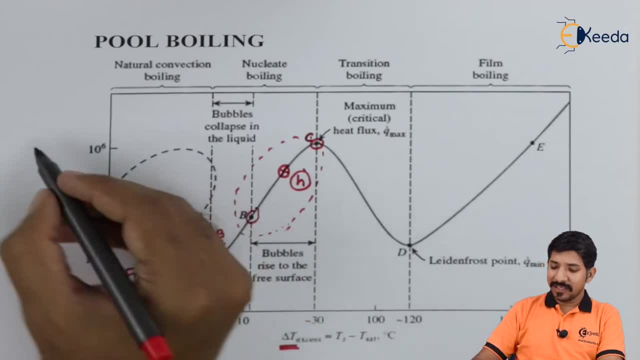 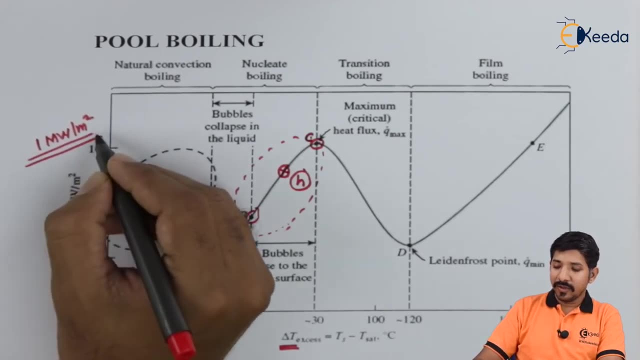 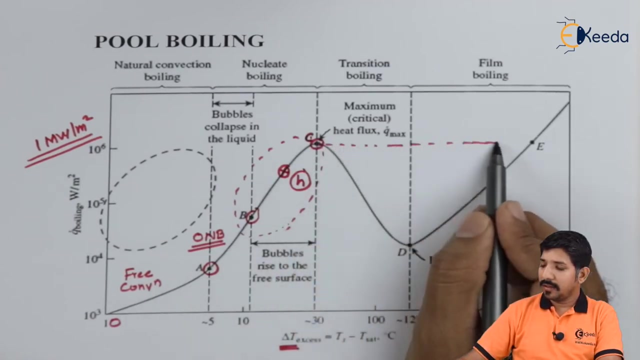 the value of this heat flux reaches around 1 megawatt per meter square. Now this is quite high, So at this value there is a possibility that the fluid or the temperature may get shoot up. so the temperature of the fluid will follow this kind of profile, so it will start from here and it may reach. 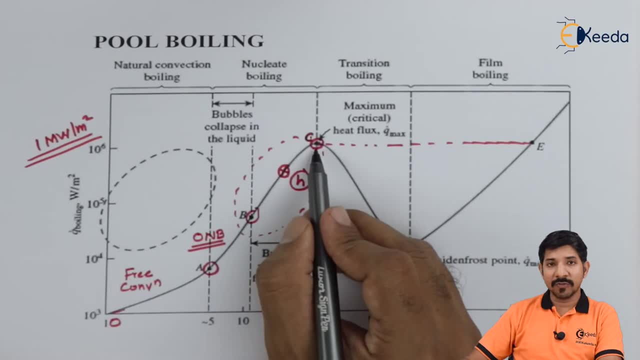 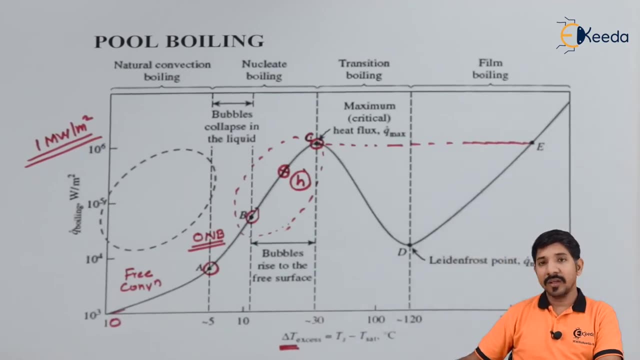 straight away somewhere here. so from delta t equal to 30 it can suddenly reach without increase in the heat transfer rate. it can suddenly reach and reach to the 1000. so now this can be a melting point of a given material. so they call this as a critical heat flux. so we don't want this point. 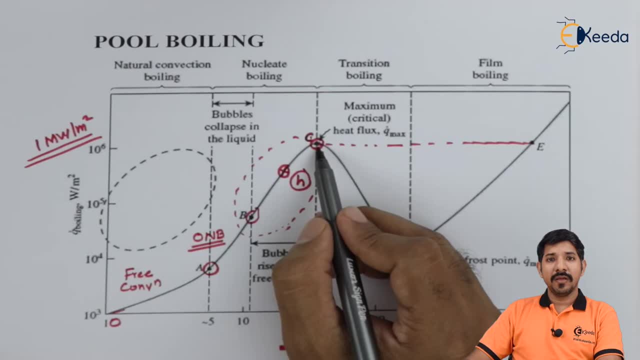 to be reached, because this point may give us the burnout. so the burnout is nothing but the melting of the given surface. so we try to avoid to this region. we try, we will make sure that the critical heat flux is not occurred. but what we want is the heat transfer rate. 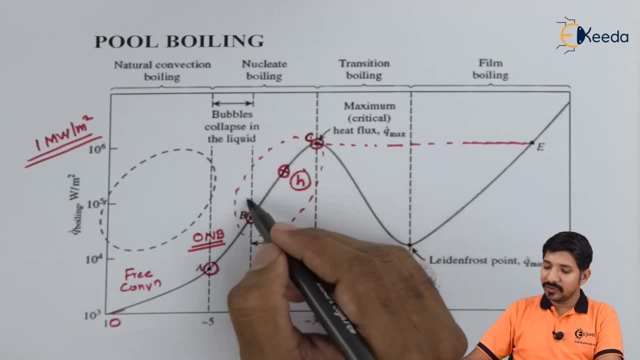 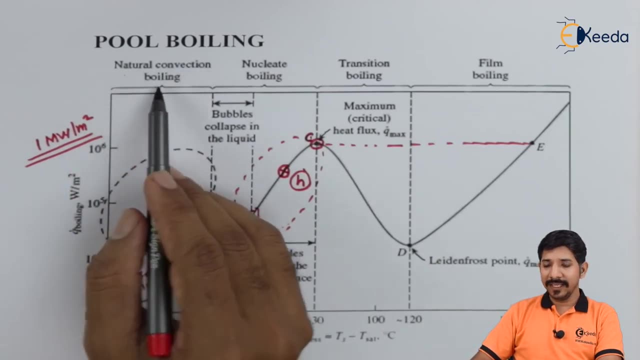 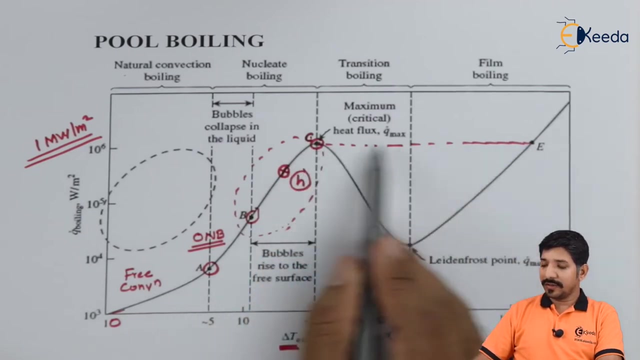 to be maximum, and that is why we need to be stayed in this region. now this is all about the nucleate boiling. we have talked about the natural convection boiling and nucleate boiling. now, if suppose the chf is not occurred, then what happens? then again, the next region that is form. 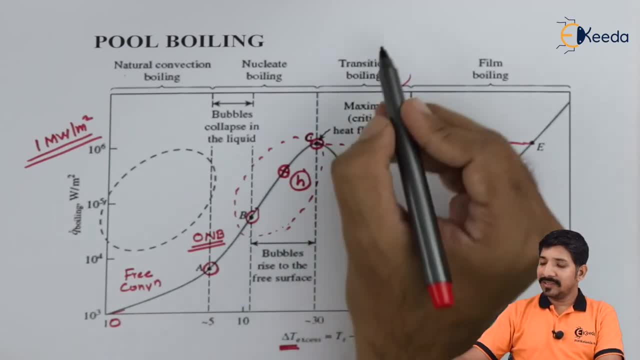 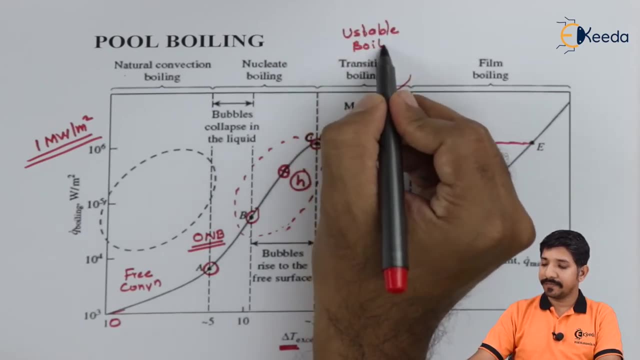 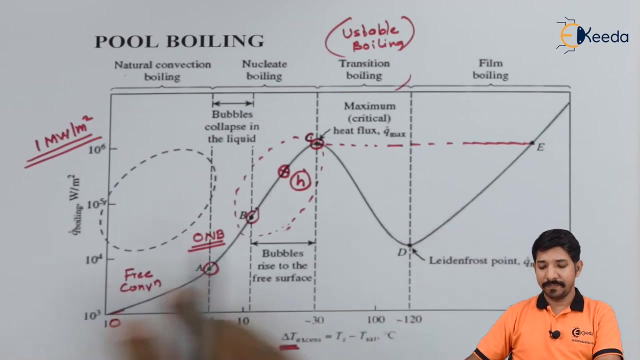 is the transition boiling. now, what do you mean by the transition boiling? this is the other name for the transition boiling- is unstable boiling. now, in case of unstable boiling, basically there is no stable film that is formed from this diagram. this part is a transition film boiling, wherein there 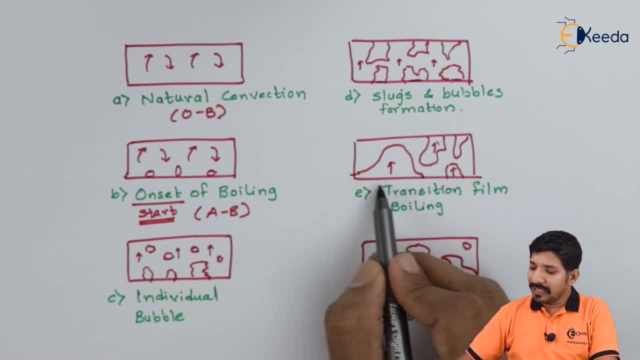 is no as such entire film. that is formed here. see only this part. the film is formed and it is not so over here. so basically, the film is not formed entirely. now, what is happening because of this? now, because of this, the heat transfer rate will suddenly drop, even if i increase the delta t. 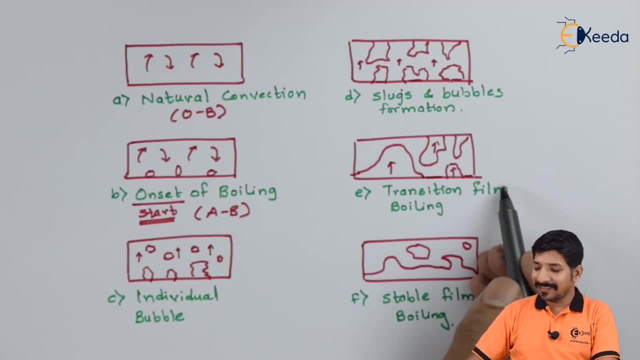 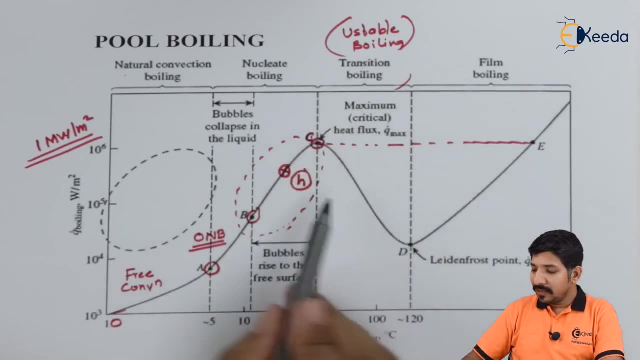 my heat transfer rate, that is, the value of h because of the lesser surface, has suddenly dropped. see, as you can see, this is the transition film boiling, or transition boiling. the heat transfer rate has suddenly dropped now, as we have seen. one more point. let us call this point as a d. so now this d comes around at: 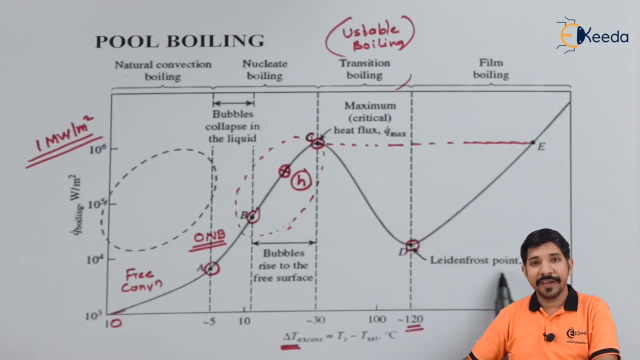 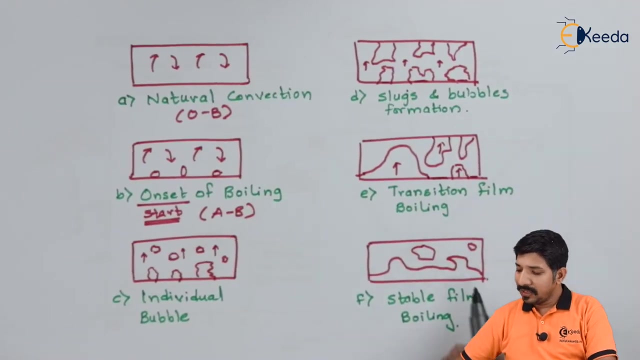 120 degree celsius. now, this d point is what they call as the latent force point. now, this is a very important point that to be understood here, so let us talk about this later. now. what comes next is the film boiling. now, what is film boiling? see, it can be seen from this diagram. the film boiling is: 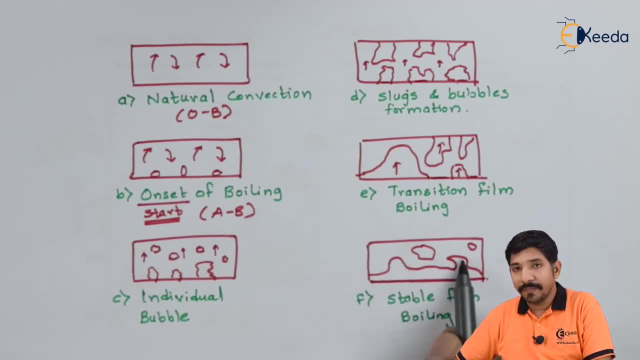 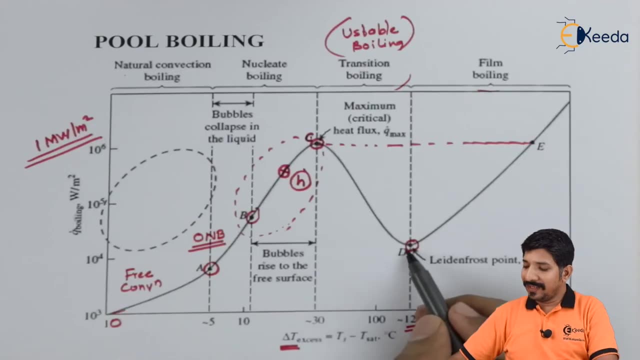 where the entire surface film. now, this film is nothing but the vapor, so it is entirely covered by the vapor itself. now, once the entire film is covered by the vapor, what is happening? due to the increased heat transfer coefficient, the value of q will again start increasing. so these were the four stages. 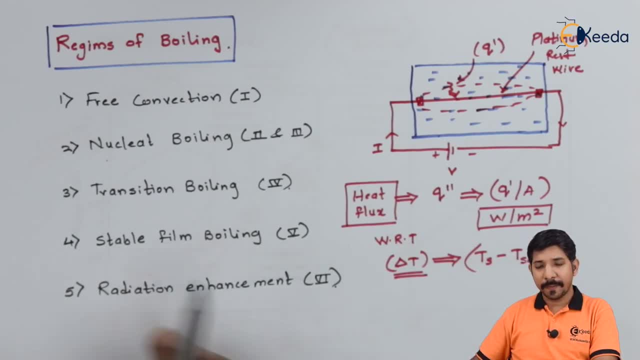 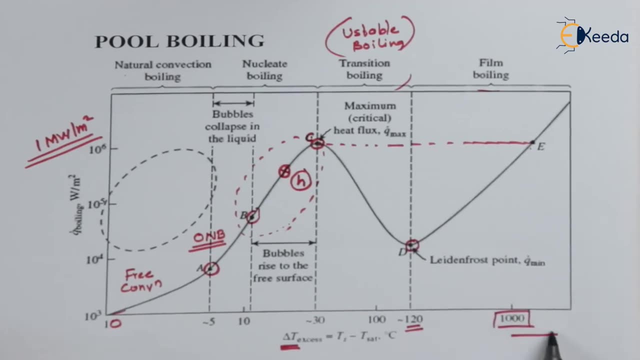 that you have seen, and the last one was the radiation enhancement. now, once i reach to a point where i have my delta t as 1000, any further increase in delta t will obviously enhance the heat transfer rate by radiation and the value of q dash will keep on increasing. now this is due. 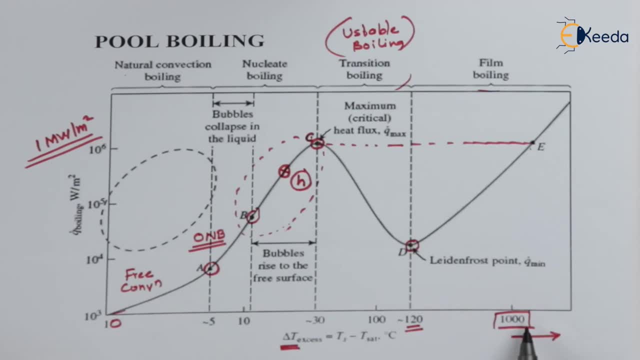 to here. after this delta t, the role of conduction and convection has decreased. it is the radiation that will be more dominant in this case. so that is all about the various boiling causes of heat transfer, as i mentioned earlier. now let's talk about the operating system more. 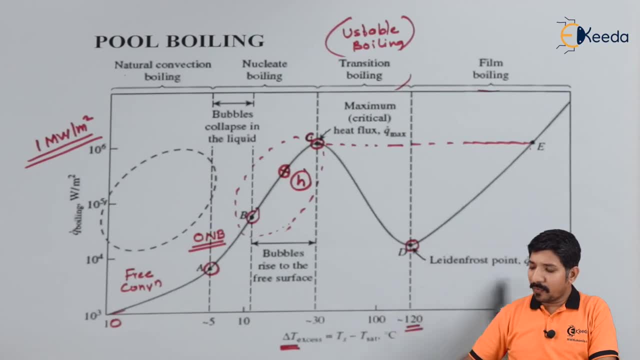 as i mentioned earlier. now let's talk about the operating system- more region- that we have studied. now let us talk about this latent frost point. now, what is the latent frost point? this latent frost point is the point where the bubbles start dancing. you might have seen while a dosa maker, so he tried to pour a small or few amount of water to check the surface. 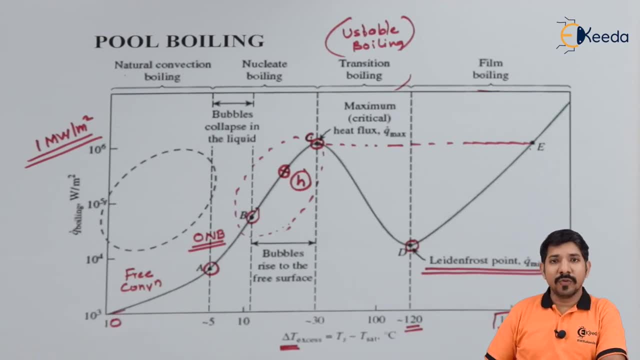 temperature of the tawa. so, basically, to check the surface temperature of the surface. what he does is he tried to sprinkle some water. so after sprinkling some amount of water, what is happening? those water droplets will start dancing over a surface or a tawa, and then it will immediately. 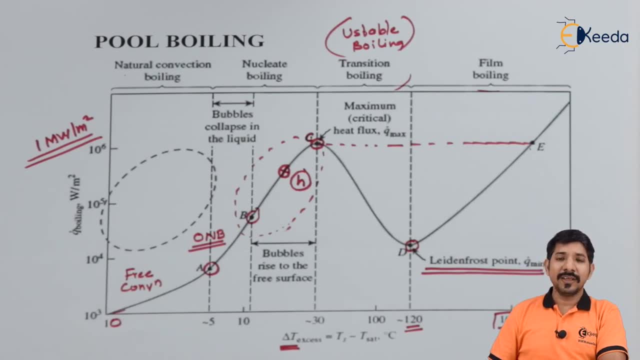 vaporize. so basically, what is happening? even though the delta t is quite high, the phase change, that is, from liquid to vapor, will not be sudden. the droplet will initially dance on the surface and then later they will get evaporated. now this point is what they call as a latent frost point, where